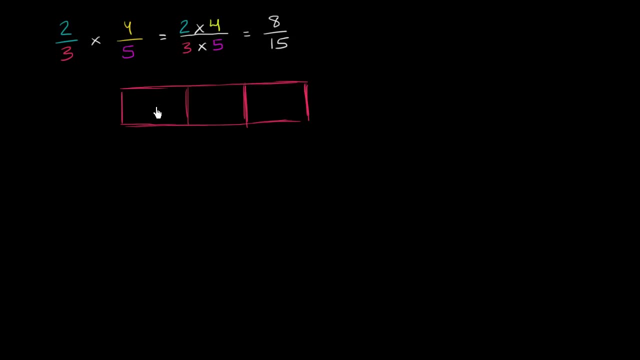 Or at least closer to looking equal. So there you go, I have thirds. Let me do it one more time. So here I have drawn thirds. 2 thirds represents 2 of them. It represents 2 of them, And one way to think about this is: this is 2 thirds times 4 fifths is 4 fifths of this 2 thirds. 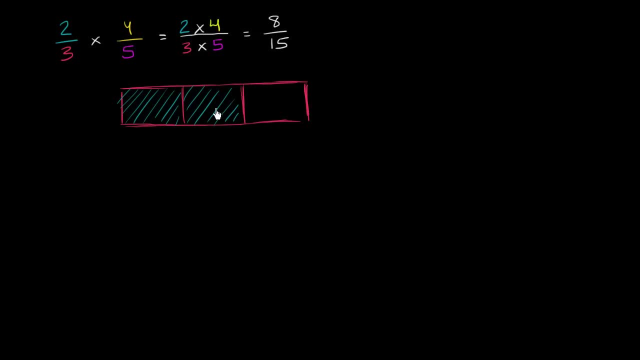 So how do we divide this 2 thirds into fifths? What if we divided each of these sections into 5?? So let's do that. So let's divide each into 5.. 1,, 2,, 3,, 4,, 5.. 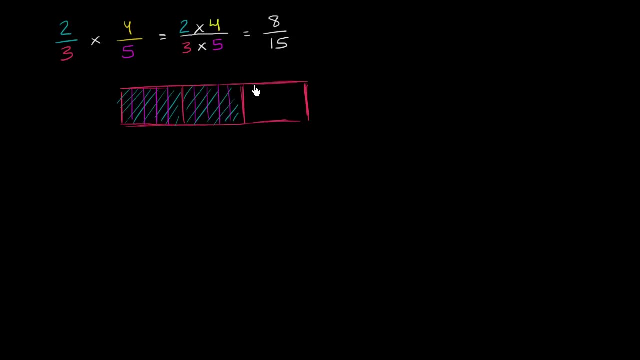 1,, 2,, 3,, 4,, 5.. And I could even divide this into 5 if I want 1,, 2,, 3,, 4, 5.. And we want to take 4 fifths of this section here. 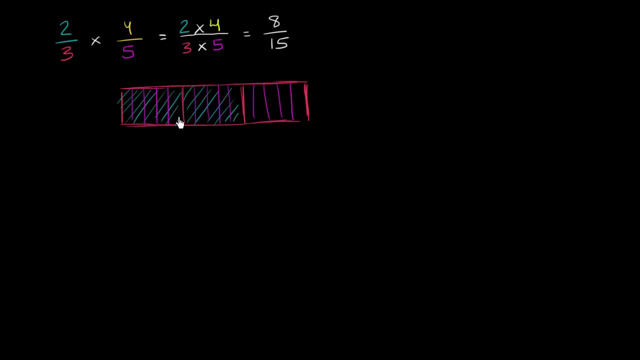 So how many fifths do we have here? We have 1,, 2,, 3,, 4,, 5,, 6,, 7,, 8,, 9,, 10.. And we've got to be careful, These really aren't fifths. 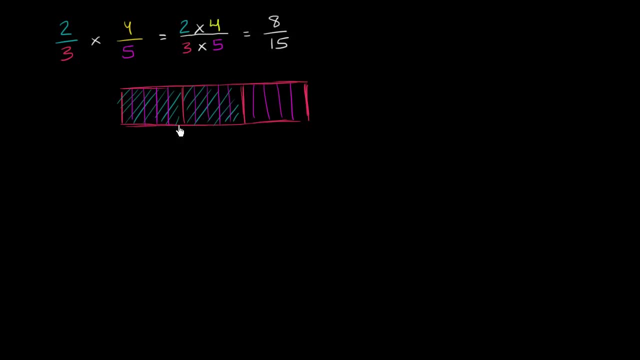 These are actually fifteenths, because the whole is this thing over here. So I should really say how many fifteenths do we have? And that's where we get this number from. But you see, you have 1, 2, 3, 4, 5, 6, 7, 8, 9, 10,, 11,, 12,, 13,, 14,, 15.. 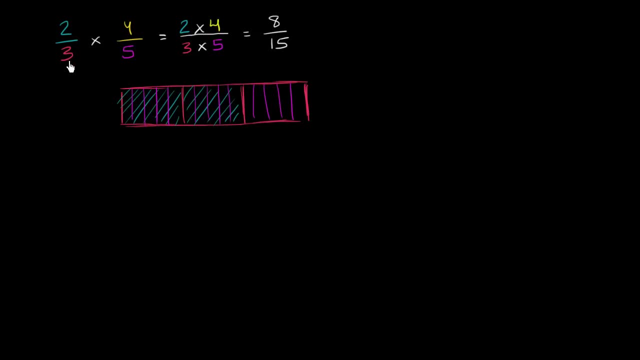 Where did that come from? I had thirds, and then I took each of those thirds and I split them into fifths. So then I had 5 times as many sections. 3 times 5 is 15.. But now we want 4 fifths. 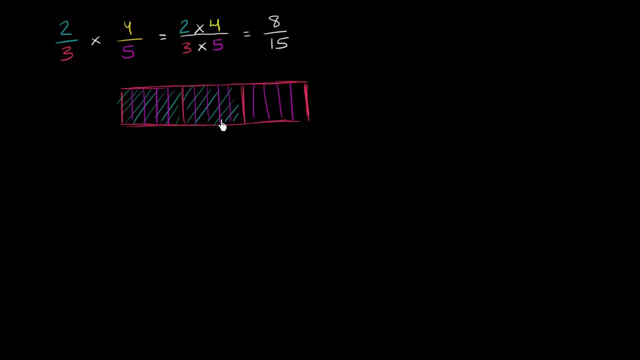 4 fifths of this right over here. So we have this is 10 fifteenths right over here. Notice that's the same thing as 2 thirds. Now, if we want to take 4 fifths of that, 4 fifths of- if you have 10 of something, that's going to be 8 of them. 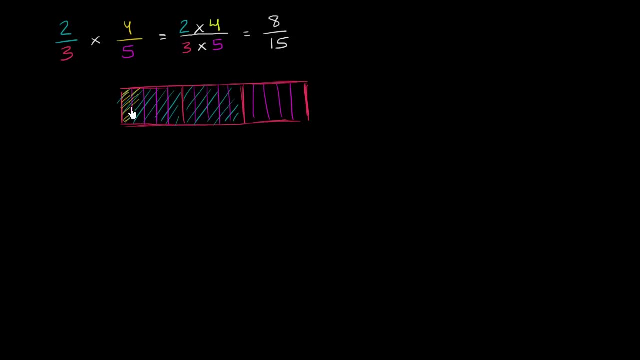 So we're going to take 8 of them. So 1, 2, 3,, 4,, 5, 6, 7, 8.. We took 8 of the 15. So that is 8 fifteenths.